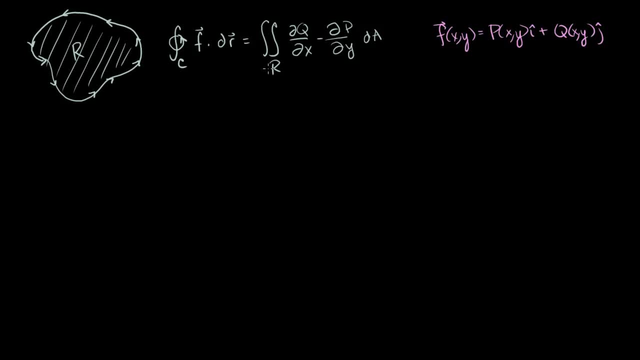 With that said, it was convenient to write Green's Theorem up here. Let's actually solve a problem. So let's say I have the line integral and let's say we're over a curve. I'll define that. I'll define the curve in a second. 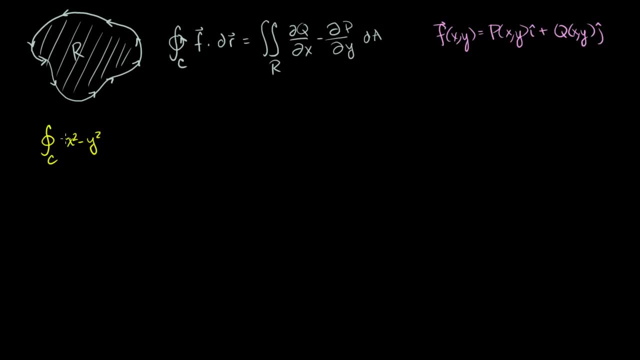 But let's say that the integral we're trying to solve is x squared minus y squared, dx plus 2xy, dy, And then our curve. they're giving us the boundary. The boundary is the region. I'll do it in a different color. 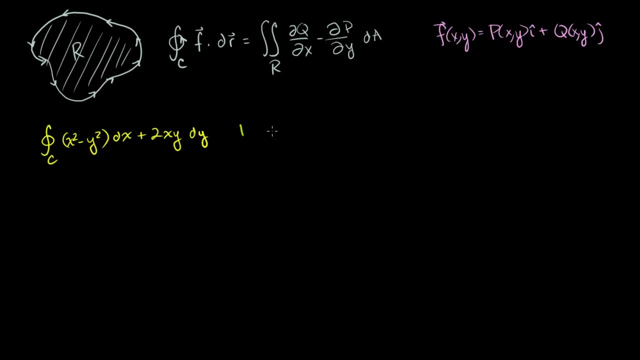 So the curve is boundary of the region given by all of the points, x, y, such that x is greater than or equal to 0, less than or equal to 1.. And then y is greater than or equal to 1.. Greater than or equal to 2x squared, and less than or equal to 2x. 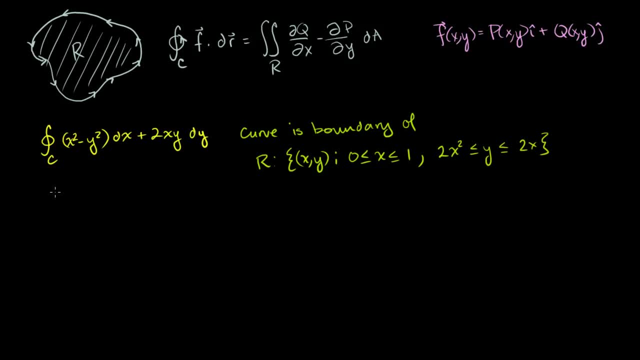 So let's draw this region that we're dealing with right now. So let me draw my y-axis and then my x-axis right there And let's see, x goes from 0 to 1.. So if we make that's obviously 0, let's say that that is. x is equal to 1.. 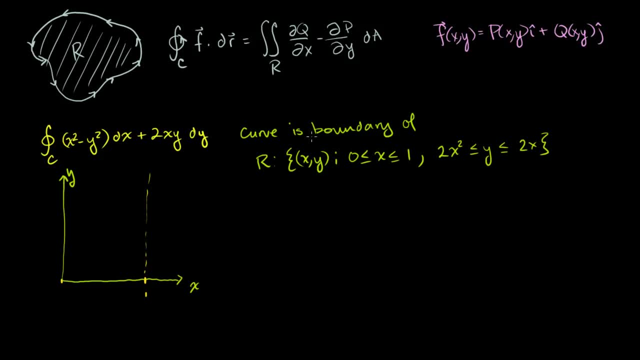 So that's all the x values And y varies. it's above 2x squared and below 2x. Normally, if you get to large enough numbers, 2x squared is larger, But if you're below 1, this is actually going to be smaller than that. 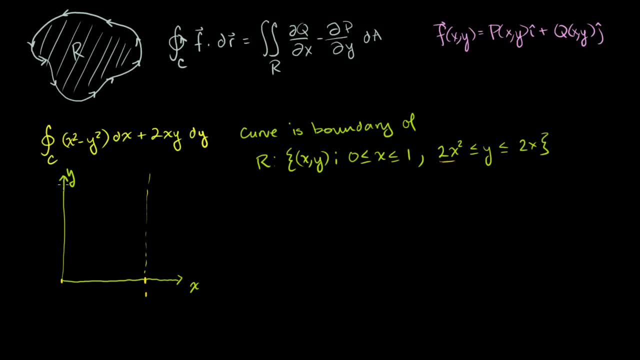 So the upper boundary is 2x. So it's 1 comma 2.. This is the line y is equal to 2x. So that is the line y is. let me draw a straighter line than that. The line y is equal to 2x looks something like that. 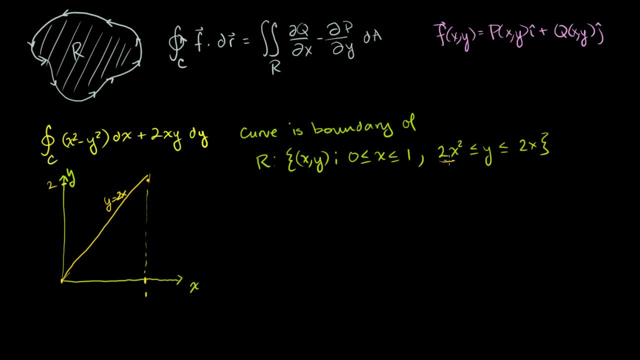 That right there There's y is equal to 2x. And then this bottom curve- maybe I'll do that in yellow- And then the bottom curve right here is y is going to be greater than 2x squared. It might look something like this: 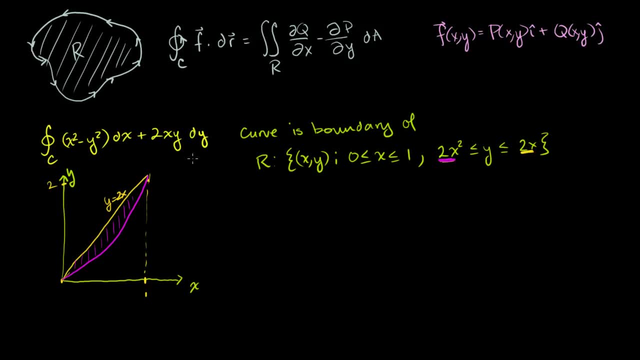 And, of course, the region that they're talking about is this. But we're saying that the curve is the boundary of this region And we're going to go in a counterclockwise direction. I have to specify that Counterclockwise direction. 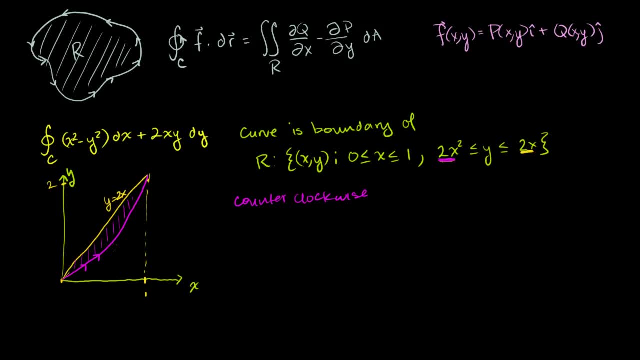 So our curve we could start at any point. We could start at any point really, But we're going to go like that and then get to that point and then come back down along that top curve, just like that. And so this met the condition that the inside of the region 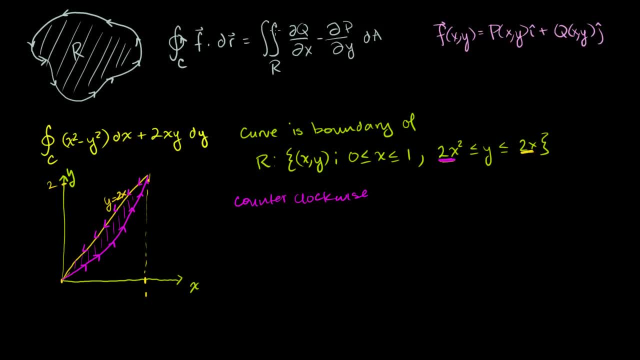 is always going to be our left. So we can just do the straight up Green's theorem, We don't have to do the negative of it, And let's define our region. So our region, let's just do our region. This integral right here is going to go. I'll just do it the way y goes from. 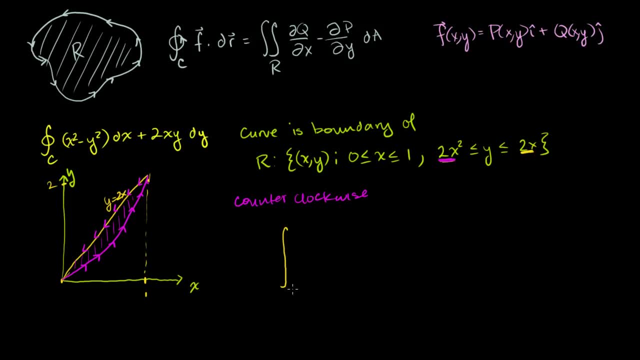 let me do it. y varies from. y is equal to 2x. squared to y is equal to 2x, And so maybe we'll integrate with respect to y first And then x. I'll do the outside. x- the boundary of x. 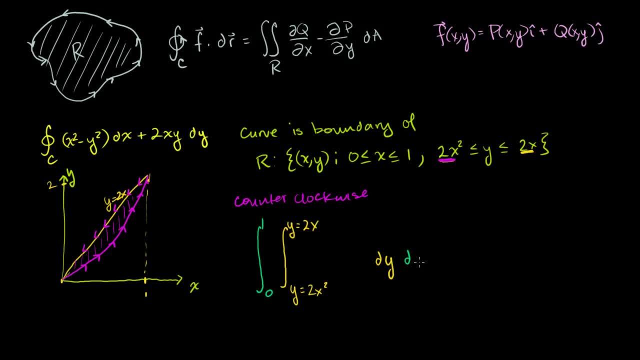 goes from 0 to 1.. So they set us up well to do an indefinite integral, And now we just have to figure out what goes over here. Green's theorem, this right here: our f would look like this in this situation: 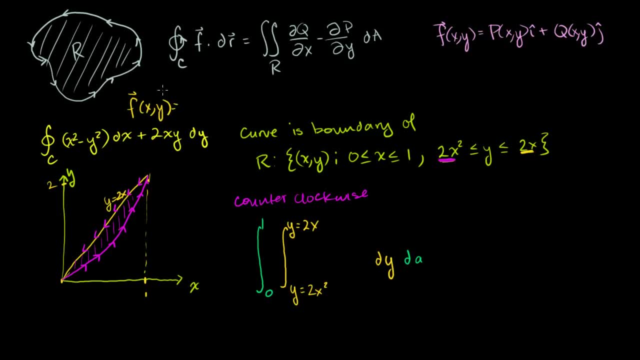 f of xy is going to be equal to x squared minus y squared i plus 2xyj. We've seen this in multiple videos. You take the dot product of this with dr. you're going to get this thing right here. So this expression right here is our p of xy. 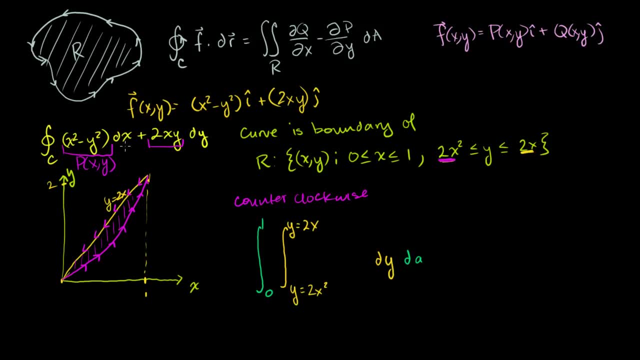 That is our p of xy and this expression right here is our q of xy. So inside of here we're just going to apply Green's theorem straight up. So the partial of q with respect to x, the partial of q with respect to x. 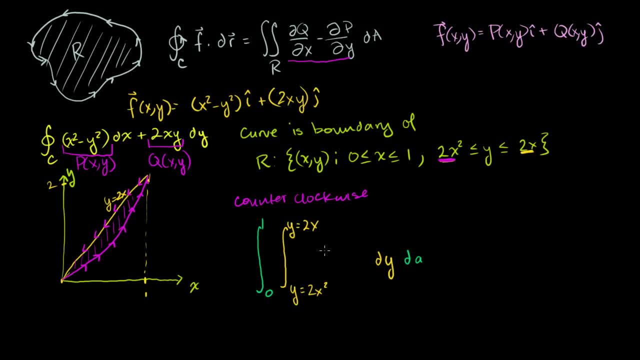 so take the derivative of this with respect to x. we're just going to end up with a 2y. So we're going to end up with a 2y And then from that we're going to subtract the partial of p with respect to y. 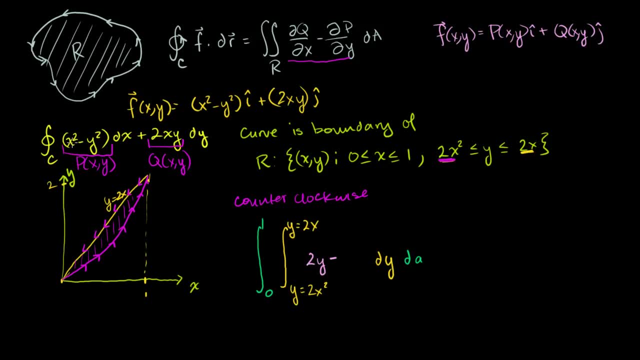 So if you take the derivative of this with respect to y, that becomes 0. And then here you have the derivative with respect to y. here is minus 2y, So you have a minus 2y, just like that. And so this simplifies to 2y minus minus 2y. 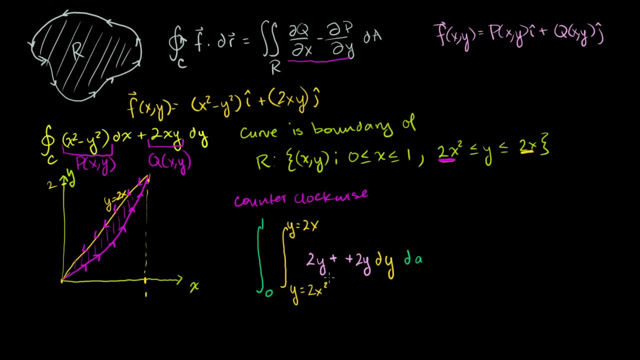 That's 2y plus plus 2y. I'm just subtracting a negative Or this inside and just to save space, this inside, let me, that's just 4y. I don't want to have to rewrite the boundaries. 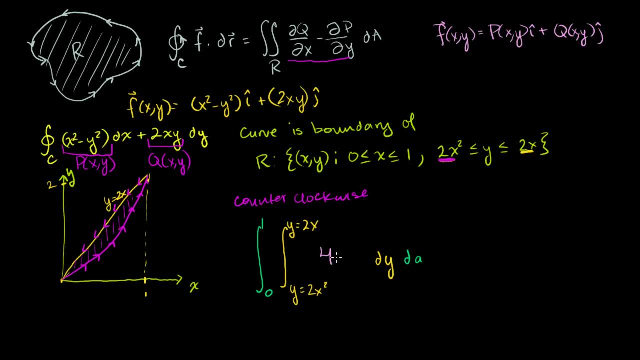 That right, there is the same thing as 4y: The partial of q with respect to y, 2y minus the partial of p with respect to y, which was minus 2y. You subtract a negative, you get a positive. you have 4y. 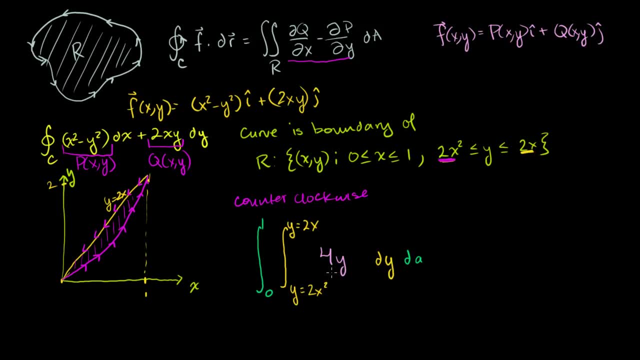 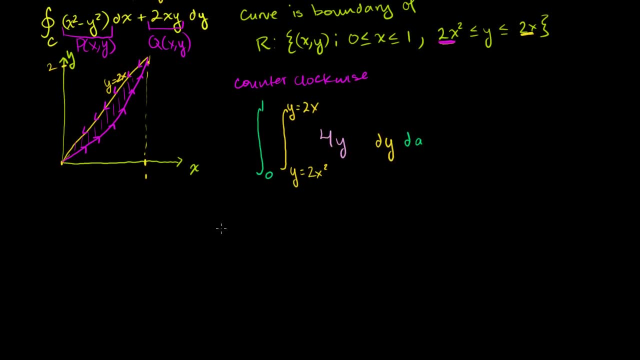 So let's take the antiderivative of the inside with respect to y And we're going to get 2y squared. Let me do it a little bit lower. We're going to get 2y squared If you take the derivative of this with respect the partial. 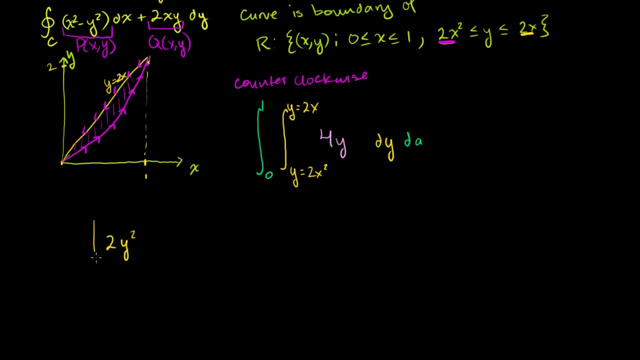 with respect to y, you're going to get 4y And we're going to evaluate that from: y is equal to 2x, squared to y is equal to 2x, And then, of course, we still have the outside integral still there. 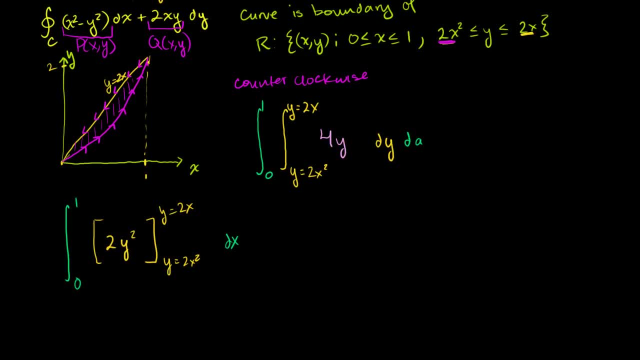 x goes from 0 to 1 dx. This thing is going to be equal to the integral from 0 to 1.. And then we evaluate it first at 2x. So you put 2x in here. 2x squared is 4x squared, right. 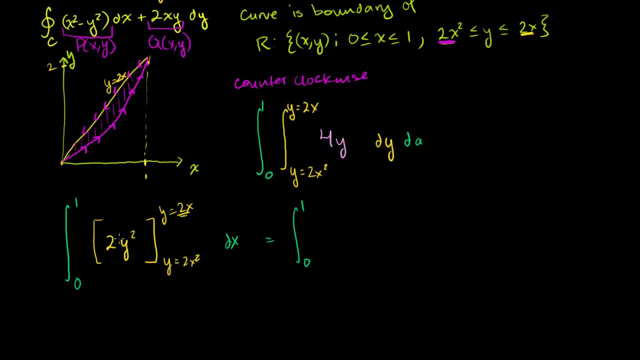 2 squared x squared, So 4x squared times 2 is going to be 8x squared minus. put this guy in there. x squared squared is 4x to the fourth times 2 is 8x to the fourth. 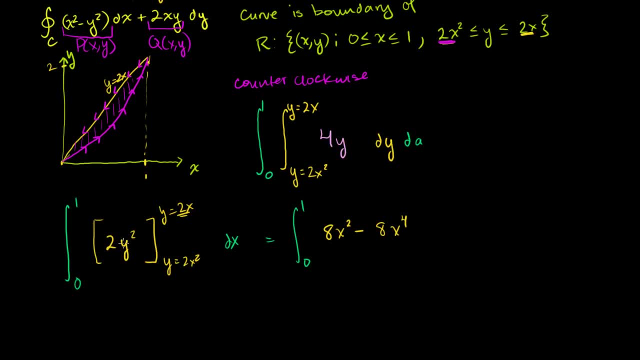 Did I do that right? 2x squared. I'm going to put it there for y, substitute y with it. that squared is 4x to the fourth times 2 is 8x to the fourth. Very good, All right. 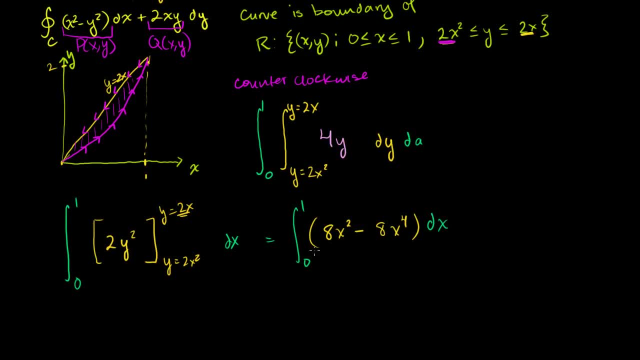 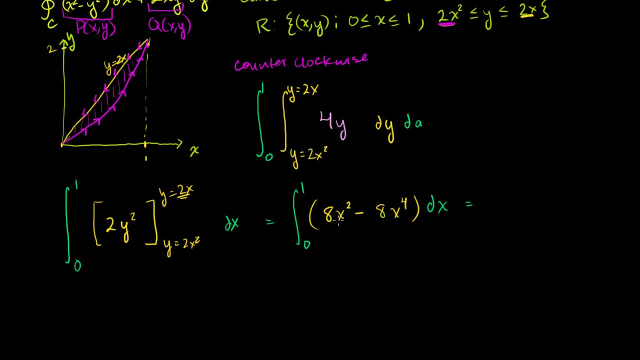 Now dx. now, this is just a straightforward one dimensional integral. This is going to be equal to- I'll just do it here: This is going to be equal to the anti-derivative of 8x. squared is 8 thirds x to the third and then the anti-derivative. 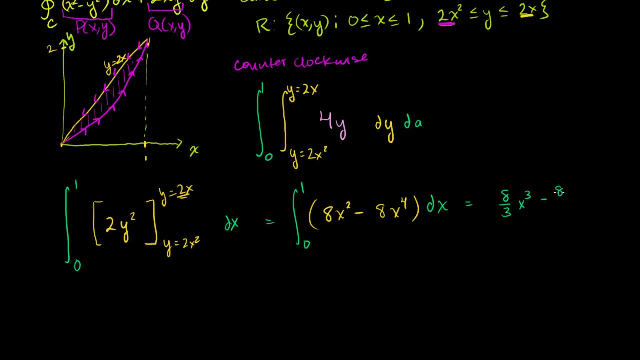 of x to the fourth is minus 8 fifths x to the fifth And we're going to have to evaluate that from 0 to 1.. I'm going to put a little line there: sometimes 0 to 1.. When you put 1 in there, you get. I'll do it in a different. 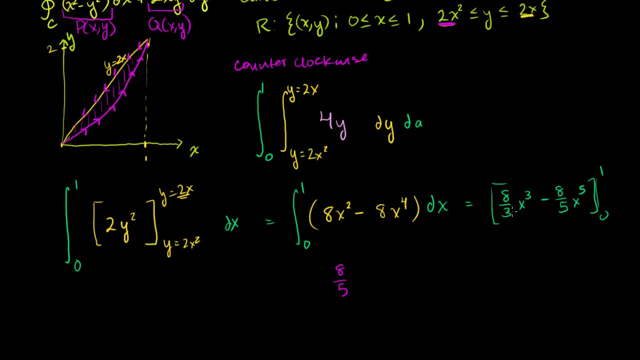 color. We get 8 fifths. I'll do it in a different color. We get 8 fifths. I'll do it in a different color. We get 8 fifths. I'll do it in a different color. Times 1 to the third, which is 8 fifths. 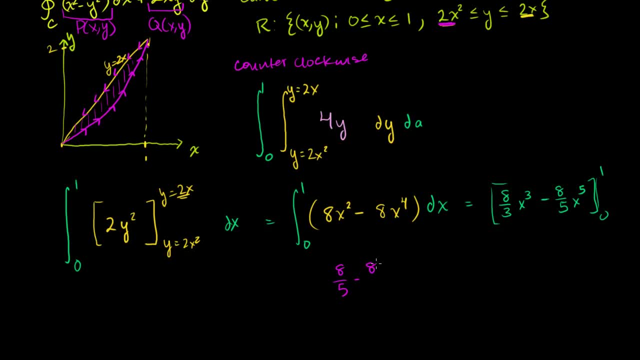 Minus 8 fifths, Minus 8 fifths, And then we're going to have minus. when you put 0 in here, you're just going to get a bunch of 0's. Oh sorry, I made a mistake. 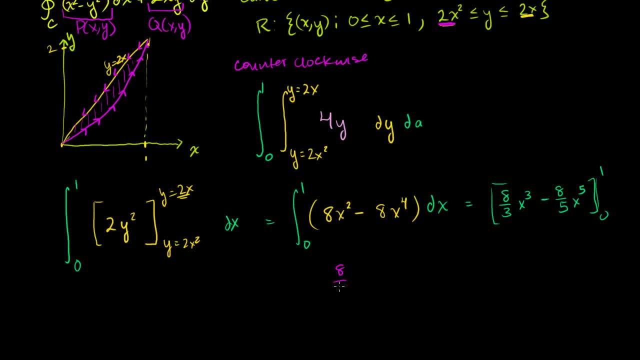 It's not a blunder, It's 8 thirds, 8 thirds, 8 thirds, times 1 to the third, Minus 8 fifths times 1 to the fifth. So that's minus 8 fifths. And then, when you subtract the 0, so then minus, you evaluate. 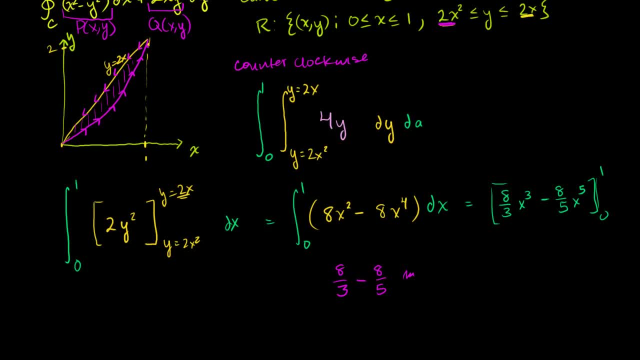 0. here you're just going to get a bunch of 0's, So you don't have to do anything else. So now we just have to subtract these two fractions, So let's get a common denominator of 15.. 8 thirds is the same thing if we multiply the numerator. 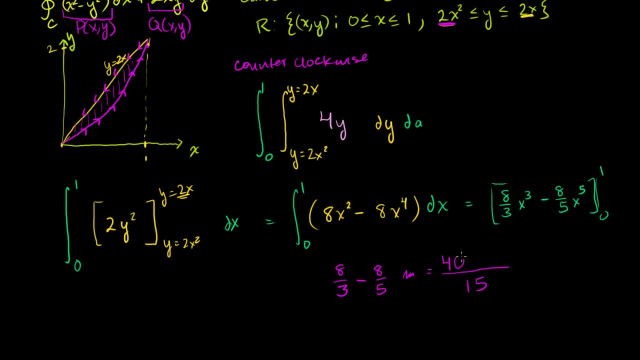 and denominator by 5. That is 40 fifteenths. And then if we multiply this numerator and denominator by 3, that's going to be 24 over 15. So minus 24 over 15. And we get it being equal to 16.. 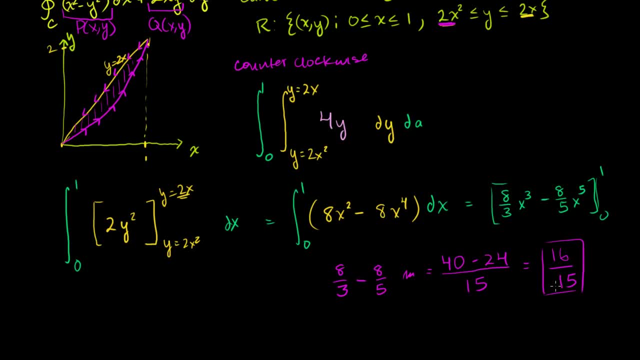 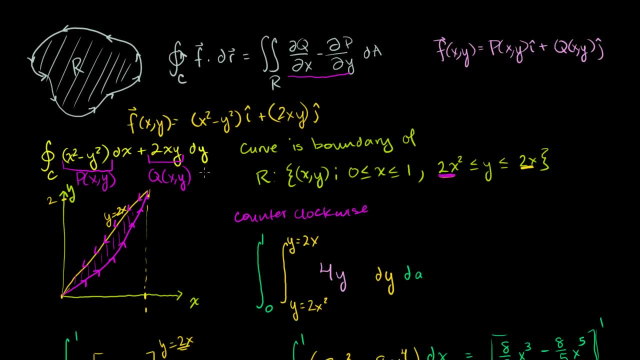 16 over 15.. And so, using Green's theorem, we were able to find the answer to this integral up here. It's equal to 16 fifteenths. Hopefully you found that useful. I'll do one more example in the next video.